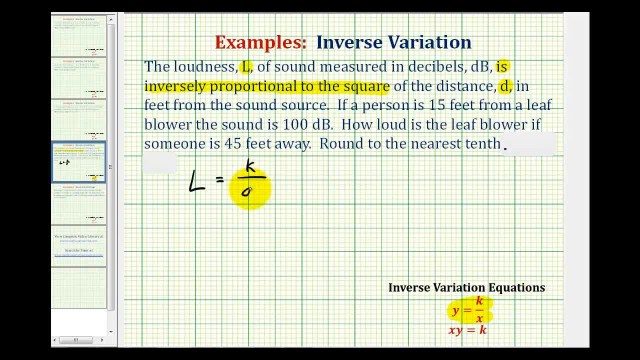 it won't just be k divided by d, it'll be k divided by d squared. And then from here we're told that if a person is fifteen feet from a leaf blower, the sound is one hundred decibels. So this is two hundred decibels. 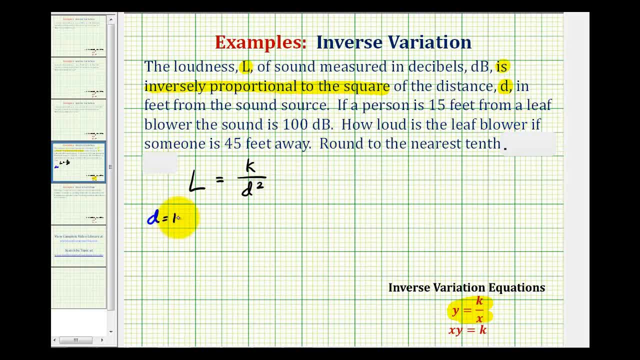 So this is telling us that if d is equal to fifteen, then L is going to be equal to one hundred. So we can use this information to find the variation constant k and then answer the question about how loud the leaf blower is from forty-five feet. 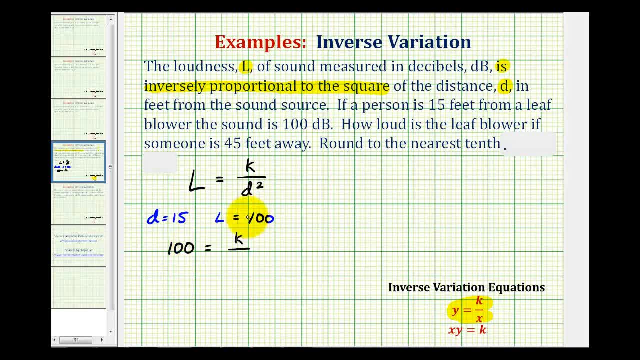 So here we'll substitute one hundred for L, But again notice, it's d squared, so we'll have fifteen squared, And fifteen squared is equal to two hundred twenty-five. One hundred equals k divided by two hundred twenty-five. Now to solve this for k, we would multiply both sides of the equation by two hundred twenty-five. 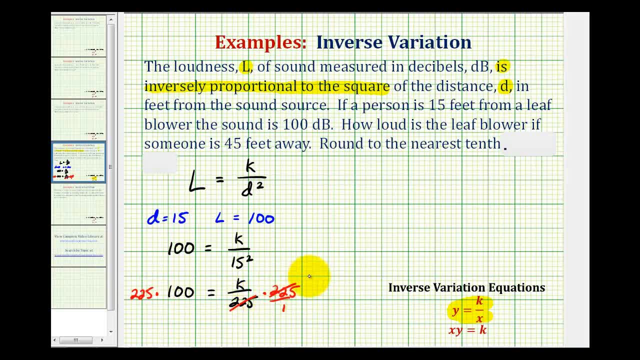 You can think of this as being over one, So this simplifies to one. So on the left side we have two hundred twenty-five times one hundred, That's going to be twenty-two thousand five hundred. On the right side we have k. 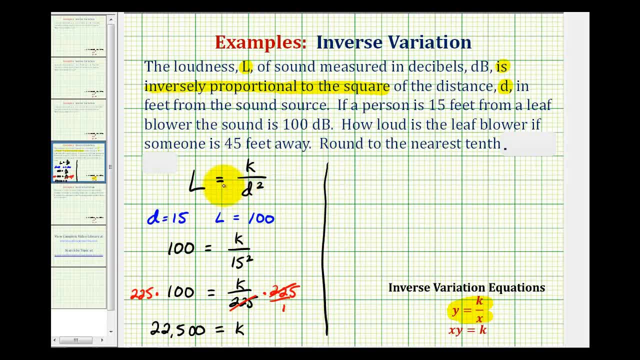 So then, for this leaf blower, the equation that relates the loudness and the distance from the leaf blower would be: L equals our variation constant, which is twenty-two thousand five hundred divided by d squared. So then, if someone is forty-five feet away, 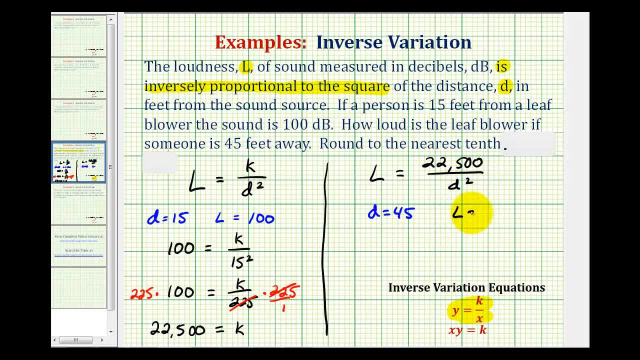 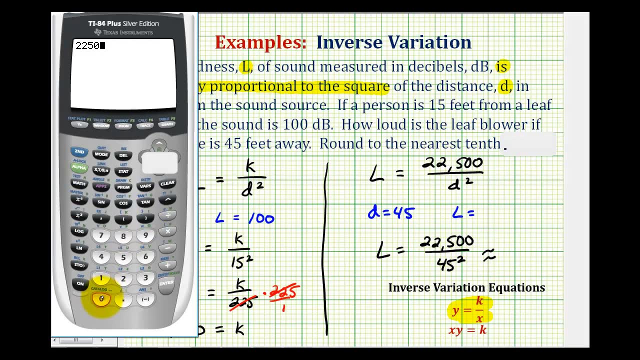 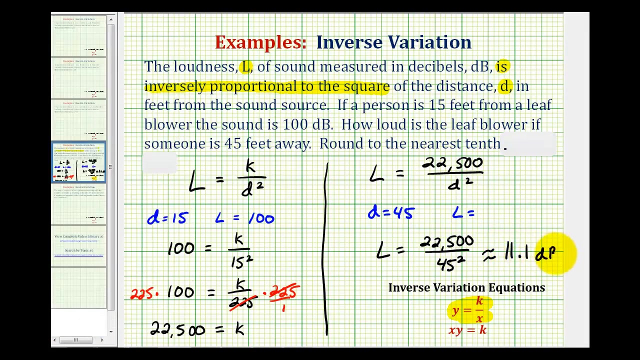 we know d is equal to forty-five. We want to determine what L would be, So we'll have: L equals twenty-two thousand five hundred divided by forty-five squared, Which would be approximately eleven point one decibels, Right into the nearest tenth. 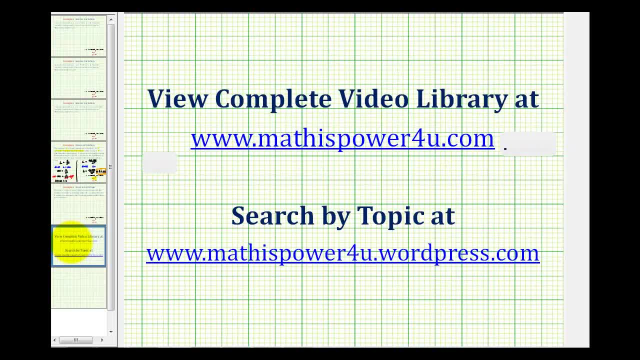 So that's everything we've got. So you can look at the equation and you can count them out. So here's our solution: We take the right-hand side and take the left-hand side. We take the left-hand side and we multiply it by two. So this's going to be one hundred twenty-five. So you take the left-hand side and you multiply it by two, And here's what we get. So now we're going to multiply this by three. So again, this is the ANS. So this is to give us the right-hand side, This is to give us the left-hand side, And we multiply this by two. So this is our sine of the power. What does that equal? 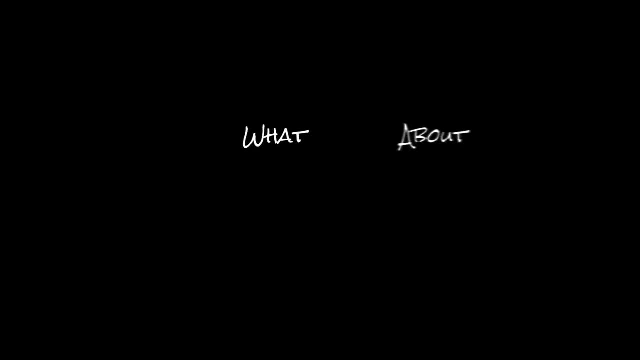 In mathematics we often solve for x, but what about y? Today I want to talk about why the Pythagorean theorem works. This is actually the third proof that I've explored on my channel, but I just think it's really cool to show multiple different paths.